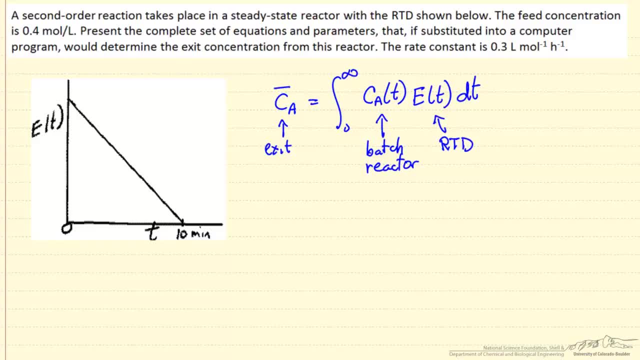 exit age distributions And we integrate from 0 to infinity. but of course in this case we only need to integrate from 0 to 10, because the diagram longer than 10 minutes. no molecules are in the reactor, So we need to do several. 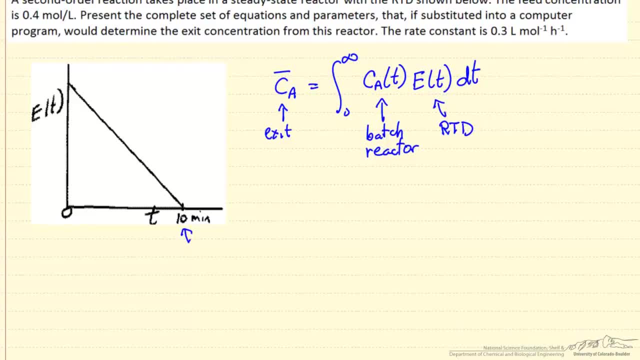 things here. First, we can determine what is e. In other words, we need the equation, we have the straight line, we need a scale for the y axis, and the way to get that is remember that the integral of e dT from 0 to infinity, or in this case, from 0 to 10,. 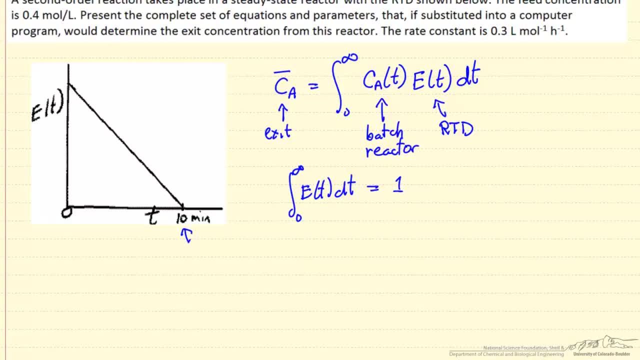 is equal to 1.. And that is the equation. We don't have to do everything. We just need to take the number of cytosine molecules and the given atomic value of chitonium, and then the corresponding have to add up to a probability of 1.. And I can make a fairly simple calculation by. 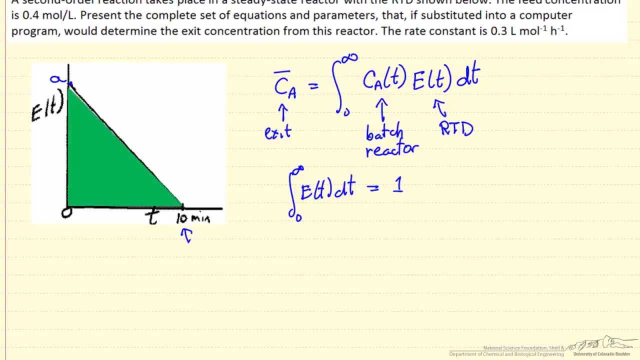 labeling this point A and saying the area of this triangle so A times 10, the x-axis times 1, half. because it's a triangle, that area should equal 1.. So A then is point 2. And this means then that our residence time distribution E of t is just a straight line. 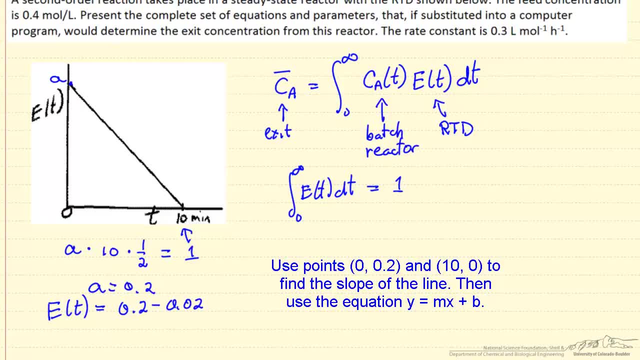 0.2 minus 0.02 times t. Batch reactor equation is just a change in concentration in the batch reactor and this is a function of time. Change in this concentration is just the rate of reaction, which is second order. So what we're going to do, we're going to solve this. 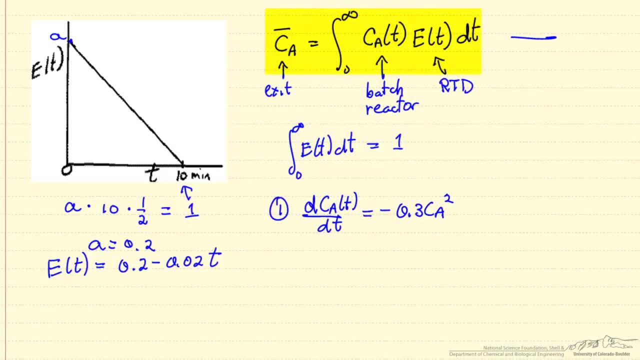 differential equation and we're going to convert this equation to a differential equation: Change in the concentration average respect to time. this will be our second differential equation, Ca, and we'll keep this function of t notation to make it clear. and then E. 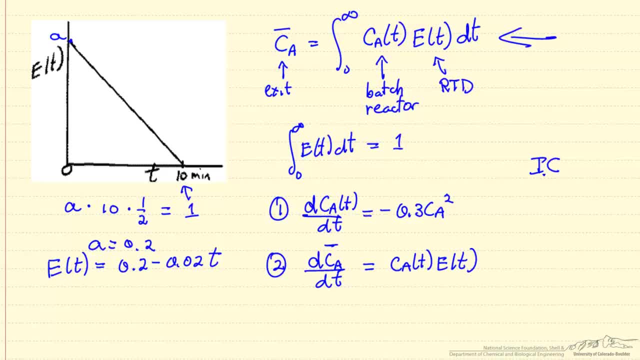 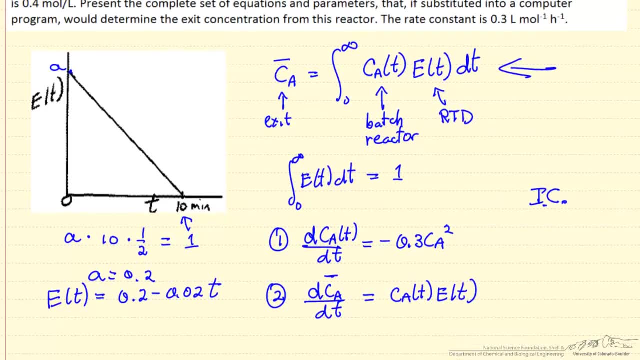 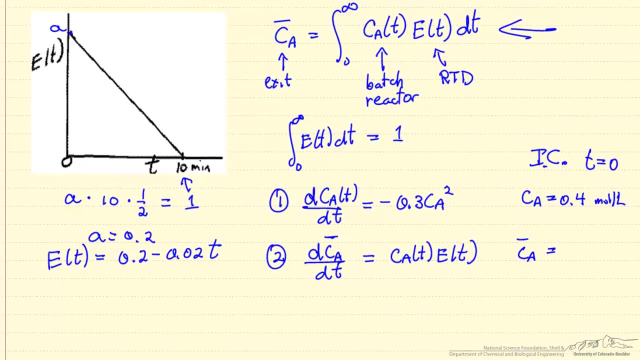 of t And we need initial conditions for these differential equations. While ca is given in the problem statement initially 0.2 by 1, and we've got the differential equation 0.4 moles per liter. this is at t equals 0, and C A average equals 0, or as we go back.